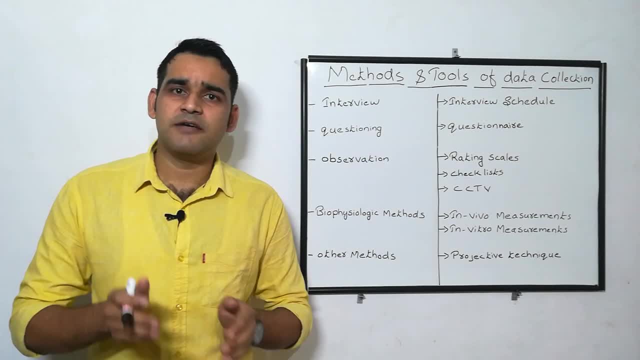 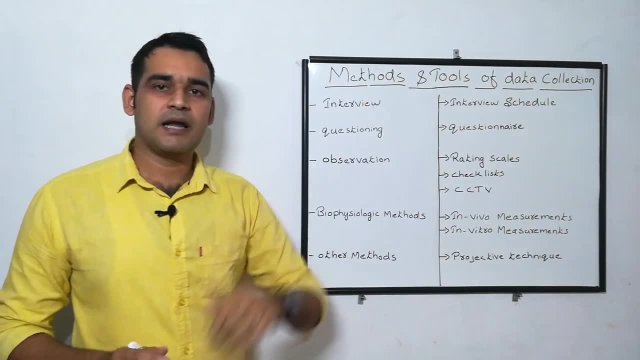 one by one. If you are referring different, different books, you will get different, different ideas. Okay, So here I have given a simple explanation regarding the methods, as well as the tools, of data collection. Let us see in detail the methods of data collection. First one is: 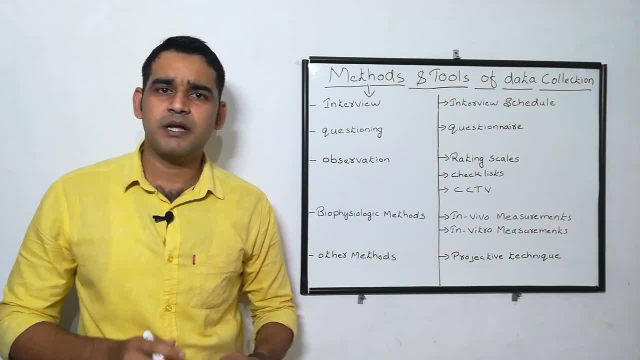 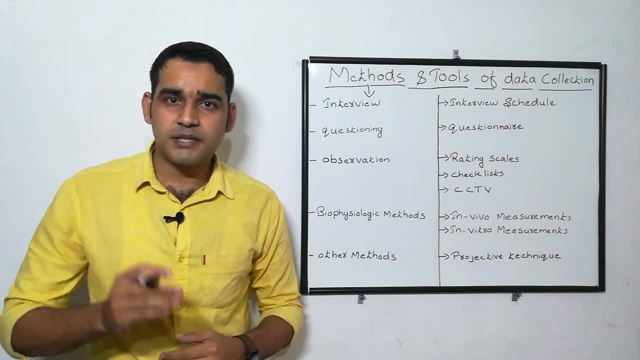 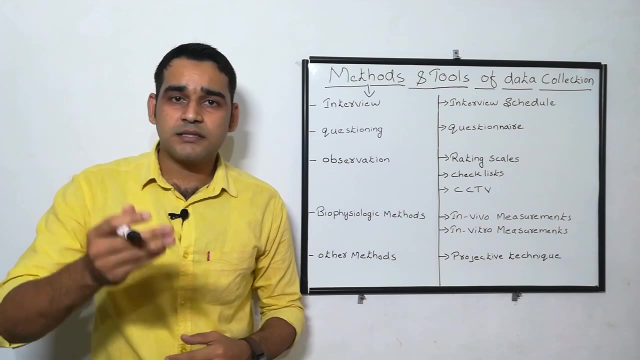 interview. First one is interview. What is mean by interview? Interview means it is a communication process, Communication process between two persons, The person. one person will ask the question and the other one will give the answer. Got it? The one who asked the? 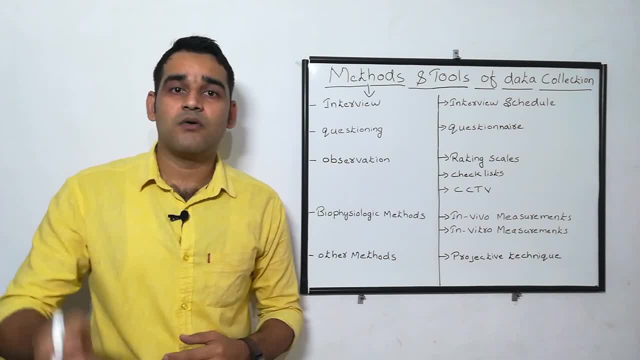 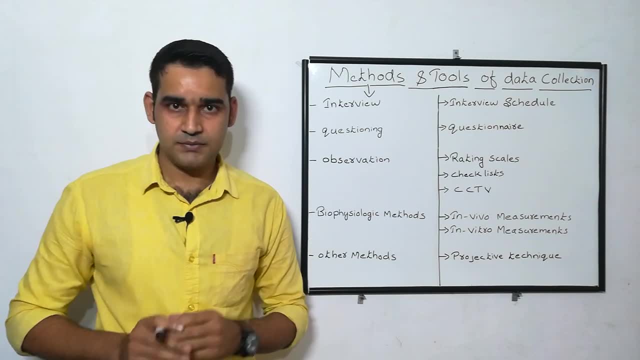 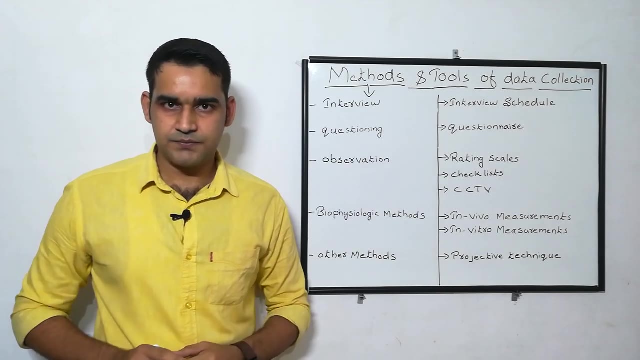 question is called the interviewer and one who give the answer is called interviewer. Got it? So it is a conversation or a communication between two persons. It is divided into interview is divided into structured interview as well as unstructured interview. Structured interview: 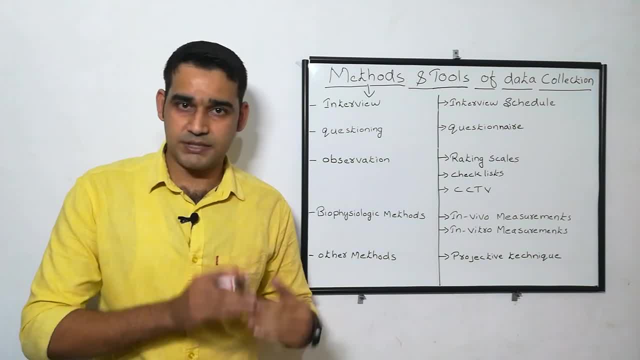 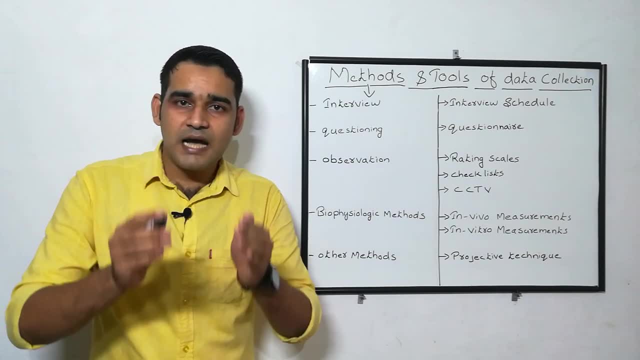 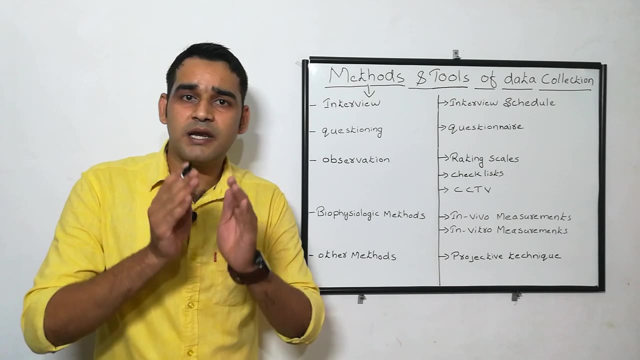 means you will have a pre-planned questions. predetermined questions will be there: 10 question or 20 questions will be there. You will ask only that: 10 questions or 20 questions according to the predetermined questions. You will ask only that You will not or you will never change the question in between. 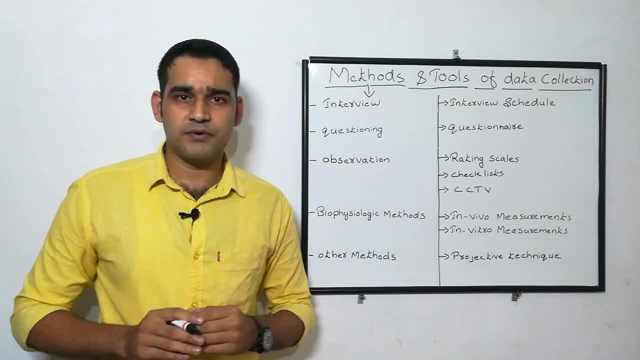 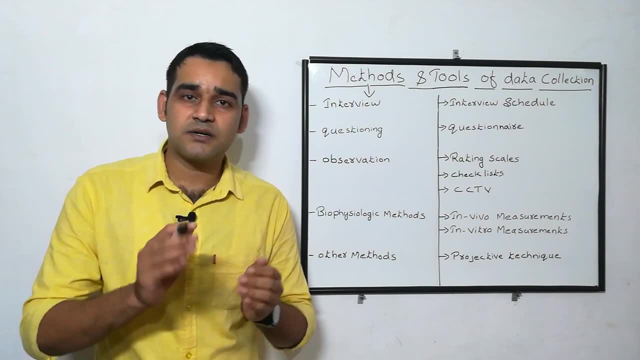 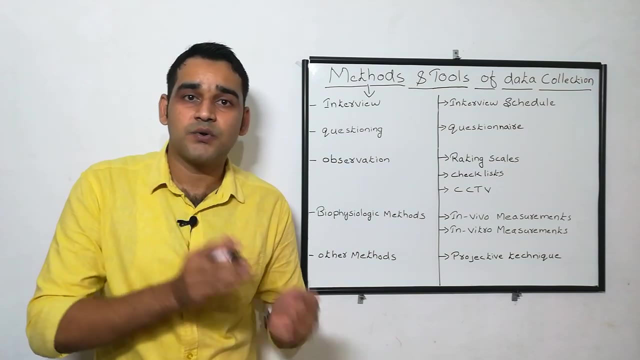 the interview. So what will be unstructured interview? Unstructured interview means just opposite to structured interview, That is, you can change the question according to the intelligent level of the interviewee, the respondent, the person who is giving the answer. You can change the questions according to the intelligence level of the respondent. 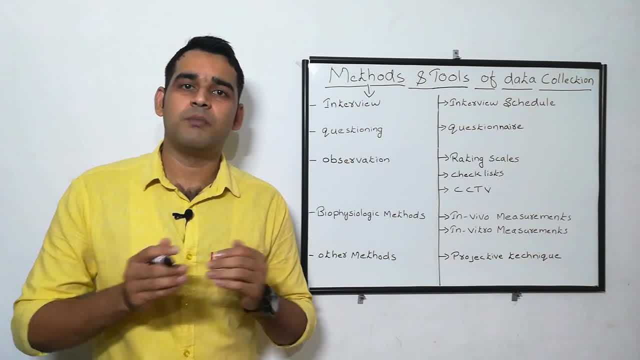 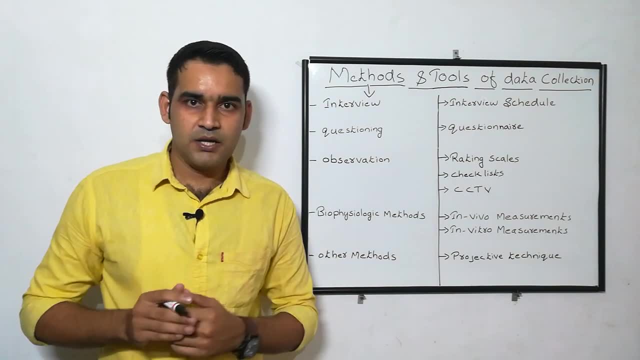 Got it. Suppose, if you are asking a question, what is your view on movement and government, If they are giving a supporting answer or a opposing answer, you can ask why. So, according to the intelligent level of the interviewee, you can change the 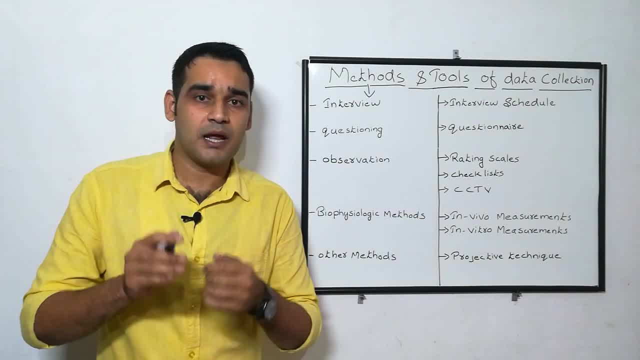 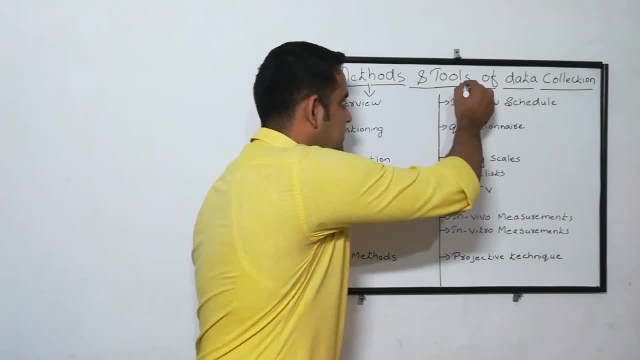 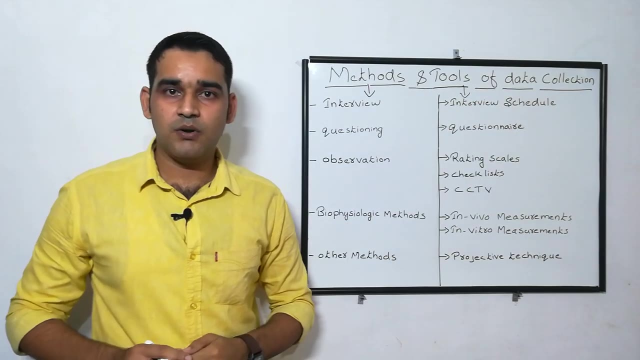 questions Here. you will not have a pre-planned questions or a predetermined question in unstructured interview, Got it? So what is the tool? The tool used for interview is interview schedule. Got it? It is interview schedule schedule. you will have a interview schedule: what to ask, when to ask, how to ask and all. 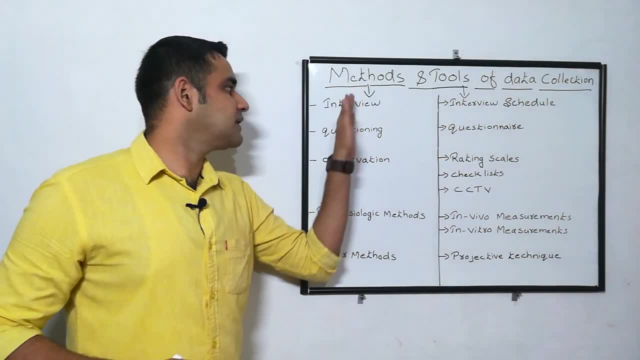 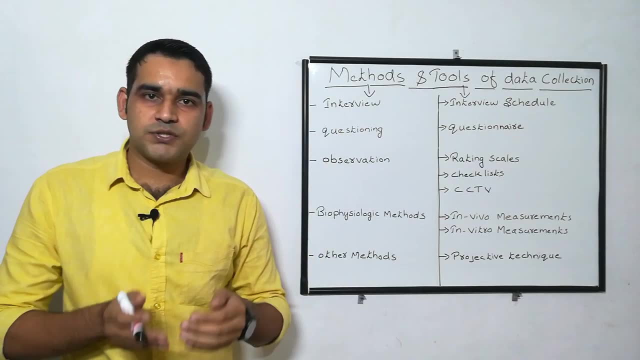 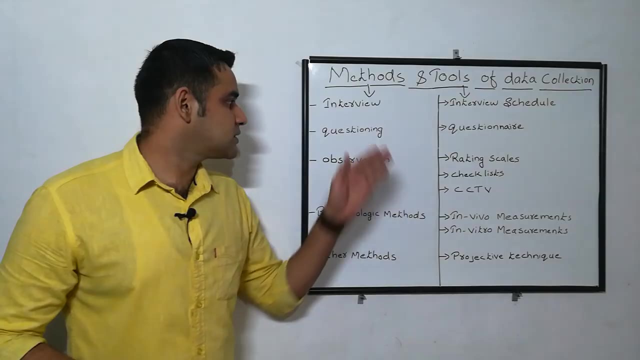 that is, interview schedule is the tool and the method is interview got it. next one is questioning. this is very familiar to you. most of the students has written exam, going to write exam right, so question paper is very familiar to you. the tool used in questioning is questionnaire. 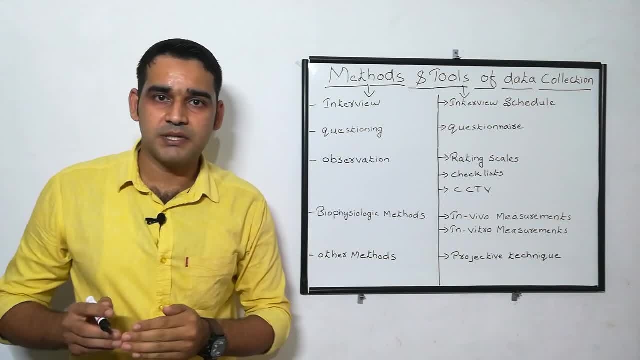 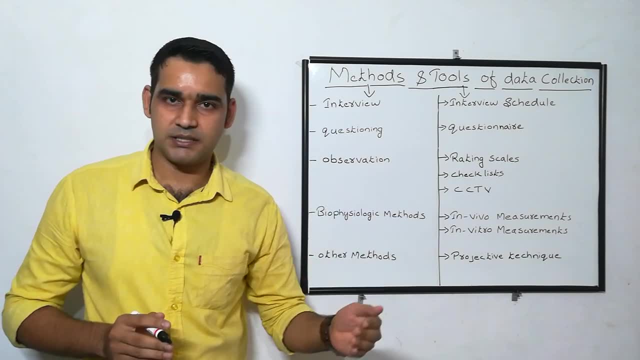 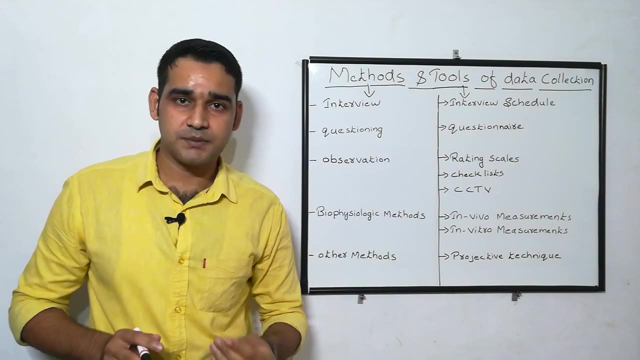 questionnaire means a series of questions will be there. it is prepared by the researcher. a series of questions will be there and the researcher will ask the subject to complete it. researcher will ask the subject to complete that question got it. it will be of two types, that is. 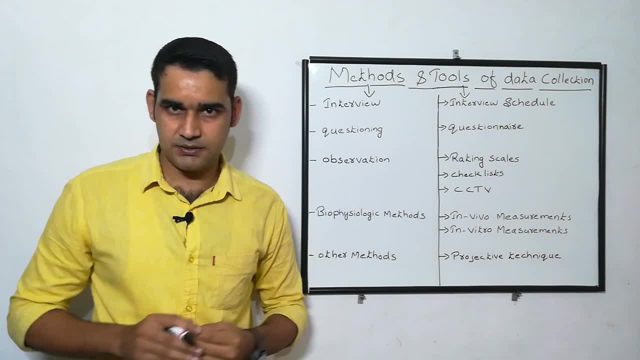 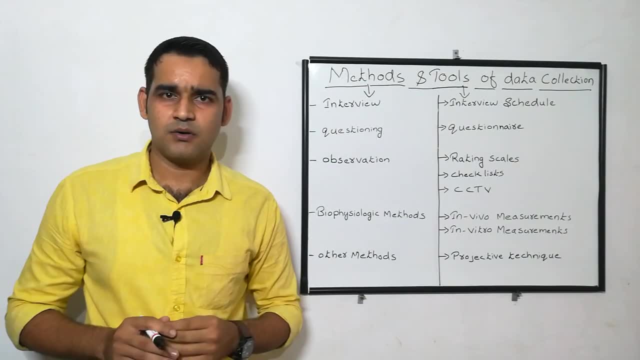 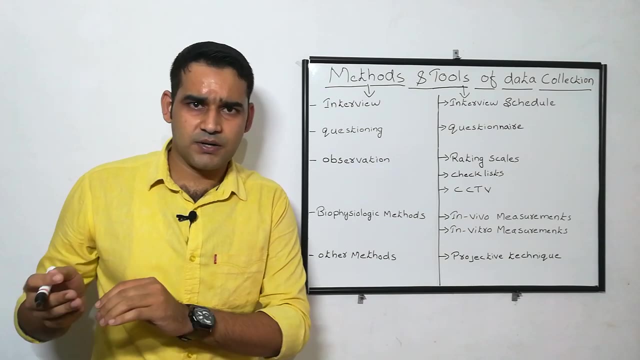 open format question as well as closed format question. open format as well as closed format question. so what is open format question means? open format question means: suppose what was the experience in that restaurant. suppose if you go to a hotel they are asking what was your experience in that? 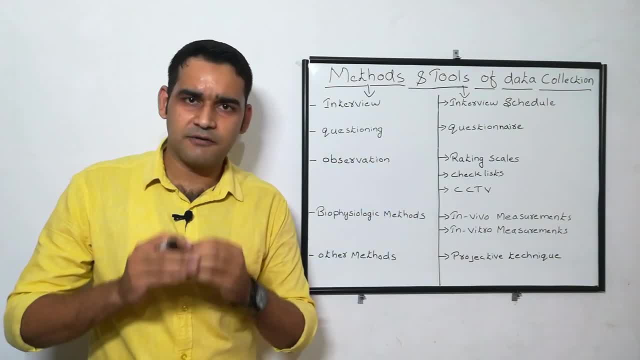 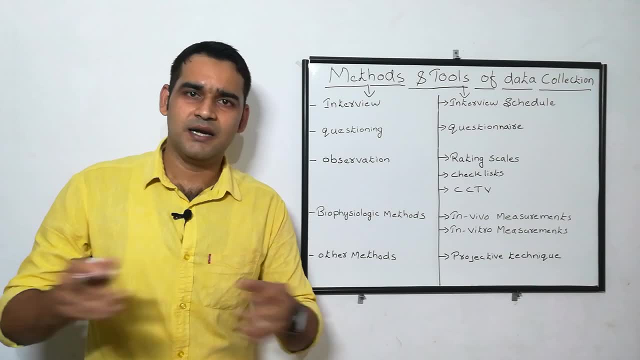 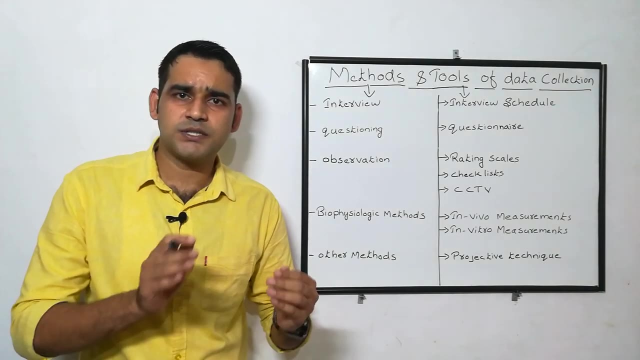 restaurant. so you can describe, regarding the food, regarding the behavior of the staff and all. you can describe this open ended in 50 words or in 100 words. you can describe in a essay manner. you can write: that is open format question. so what will be closed format? closed format means: do you like? 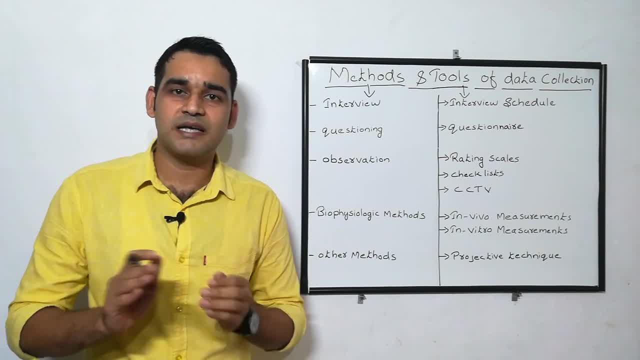 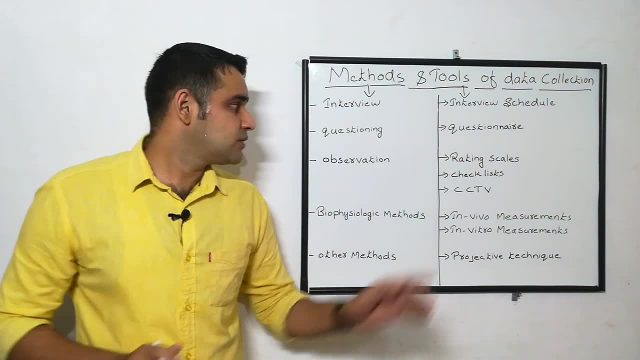 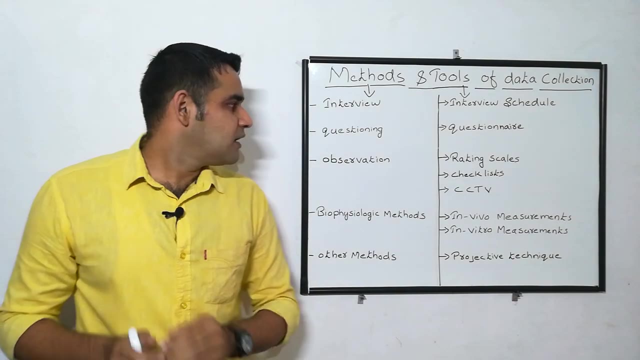 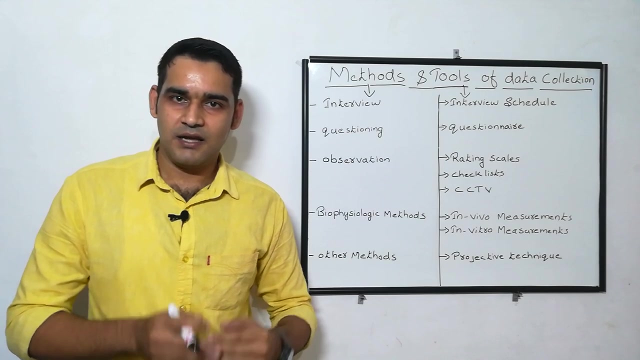 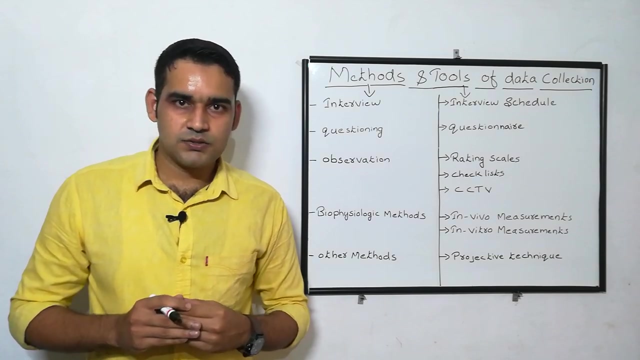 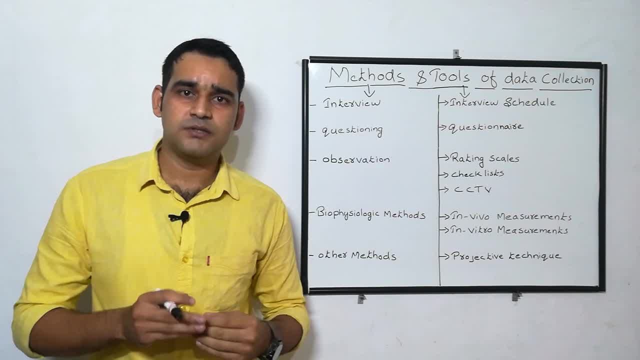 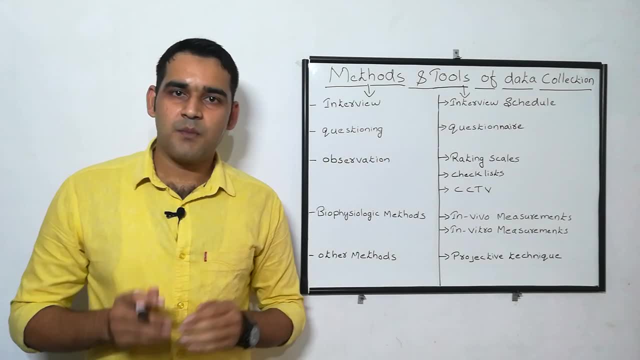 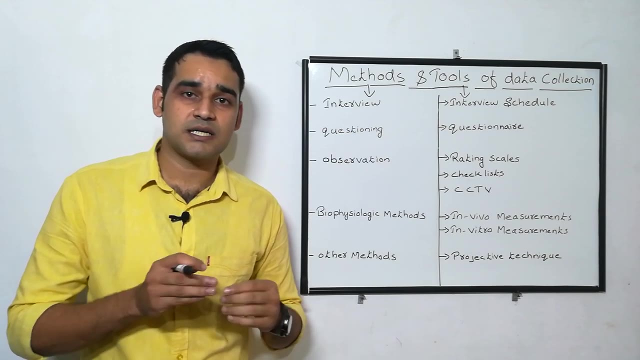 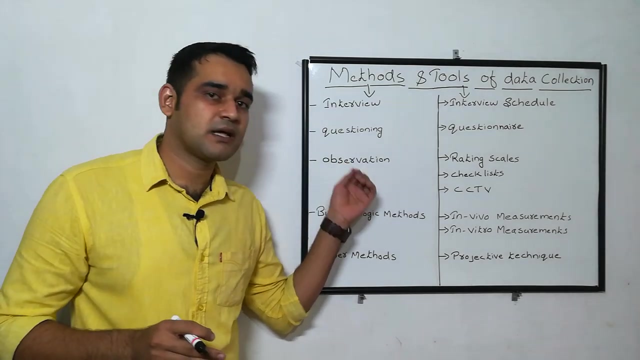 observation, participant observation and non-participant observation. observation is classified into structured observation, unstructured observation, participant observation as well as non-participant observation, got it. so what is mean by structured observation? what i have explained in interview, the types same, only here the observer, the researcher, will have a plan what to observe, when to observe, how to observe instead. 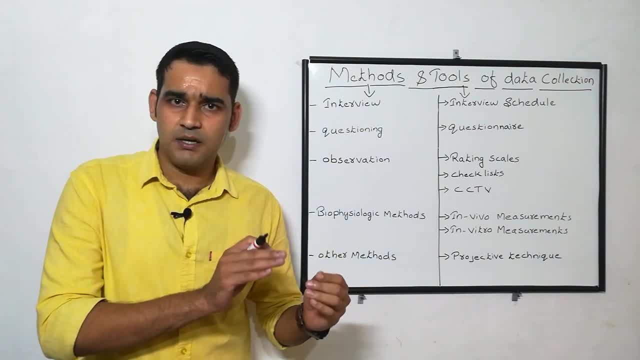 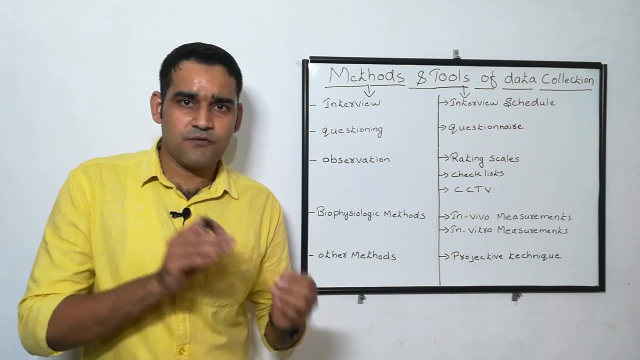 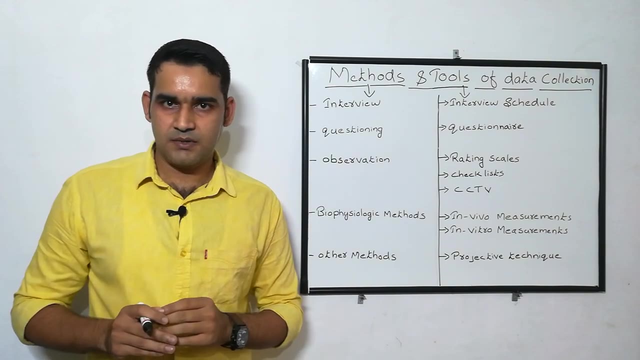 structured observation he will have a plan got it. but in unstructured observation he will not have any predetermined plan where to observe, when to observe, how to observe. he will not have any plan- just opposite to structured observation. so what is mean by participant observation? participant observation means. 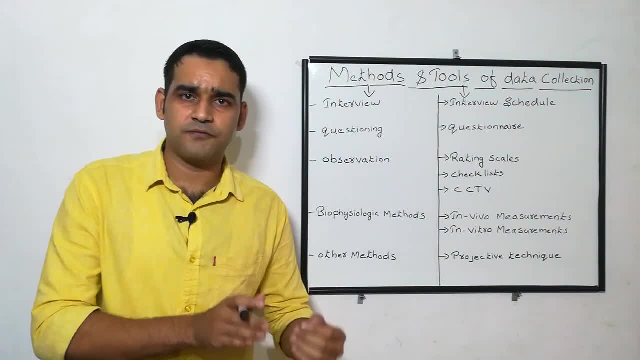 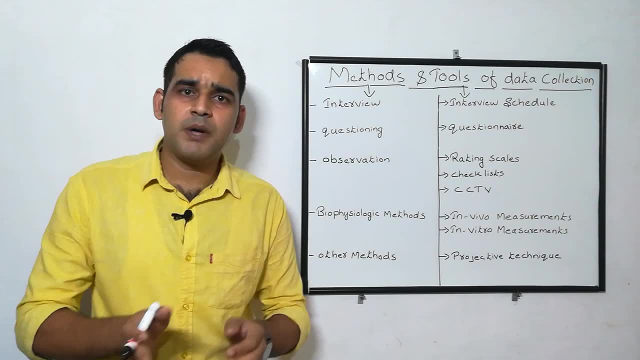 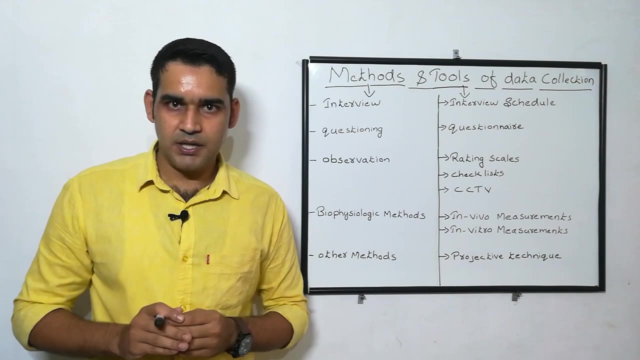 1974. 11. so what is mean by participant observation? a, when a participant object observed season, which means the observer will be a part of the event. 24- 11. so what is mean by participant observation? its want to report and quietly fly around the grade. 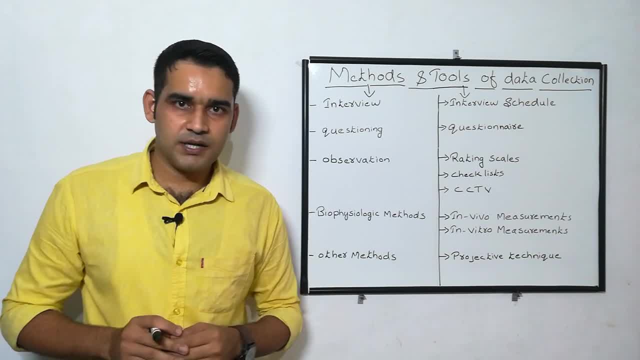 he will be a member of the team together. while playing with them with the subjects, he will obsess over things. what you want to observe, he'll be a member. he'd be a participant of that event. you, he'll be a member. he'll be a participant of that event. gotage next, hot asleep on non-participant observation. non participant observation means. antal hasn't. however, sorry. fixed setting to structure ahead of time is a partner not select every time. the ingred to develop option not become Menloing has been the travelling strategy. ways to form central espíritus happens to set certain locations, start several elements, such as Villillea, and that means five points later and ㅎㅎ. 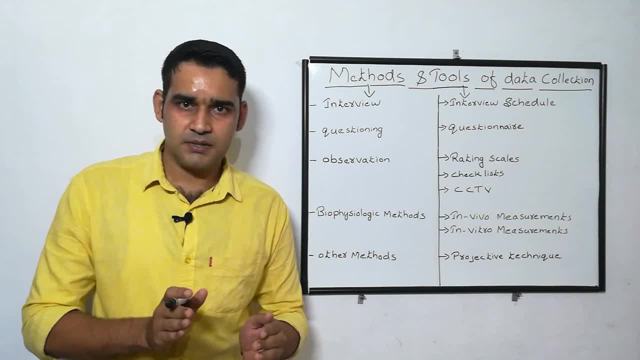 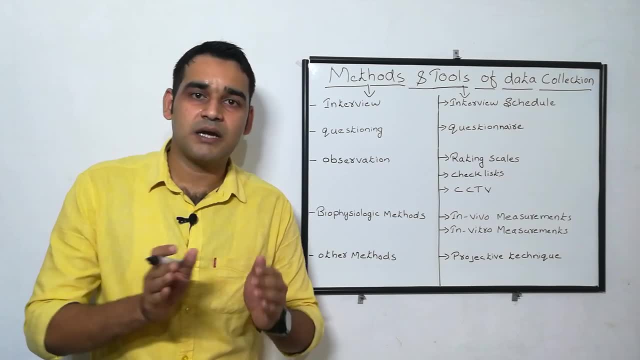 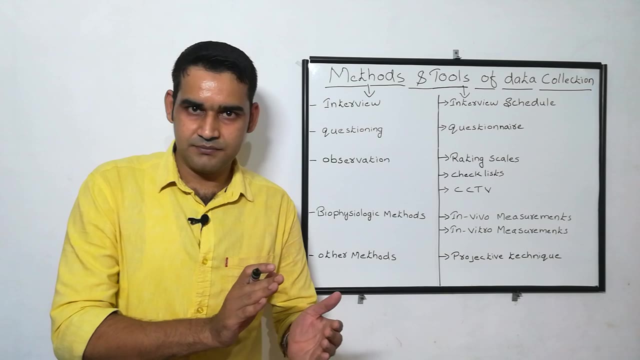 researcher will not be a part of that event. he will not participate in that. he will not participate while playing football, but in the gallery he will observe what he want to observe. got it. he is not a participant. still, his presence is there but he is not with them, got it? that is non-participant. 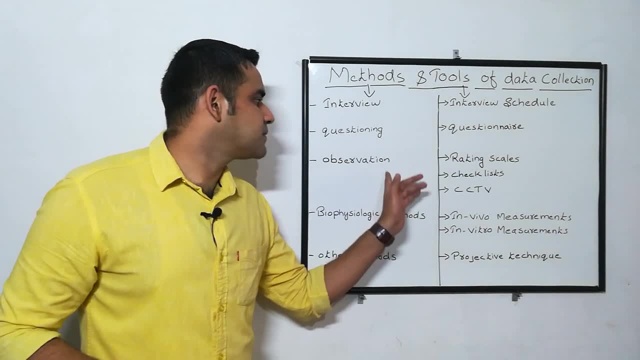 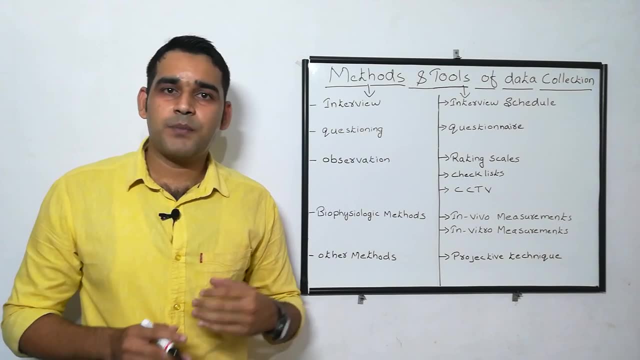 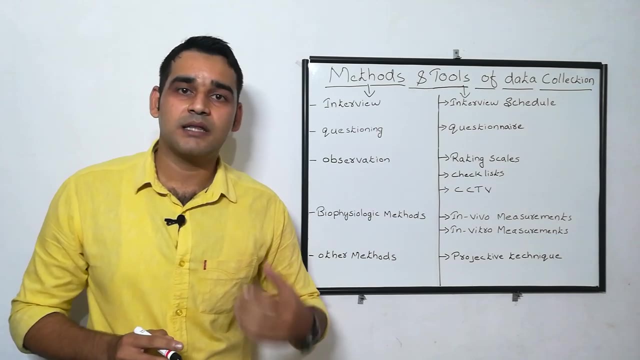 observation. so what are the tools used for observation is first, one is rating scale. rating scale means it is very familiar: nowadays, if you purchase a product from amazon or flipkart, they will ask you to write regarding the product, right regarding the service, and all got it. so the 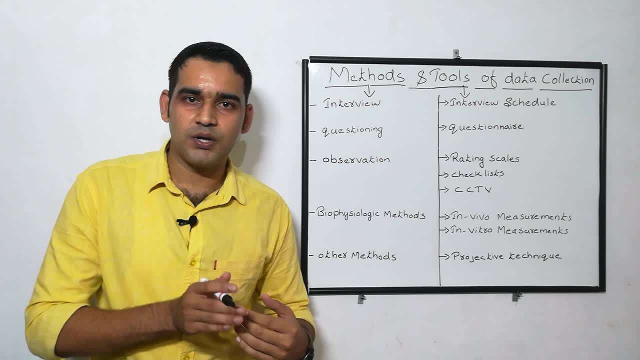 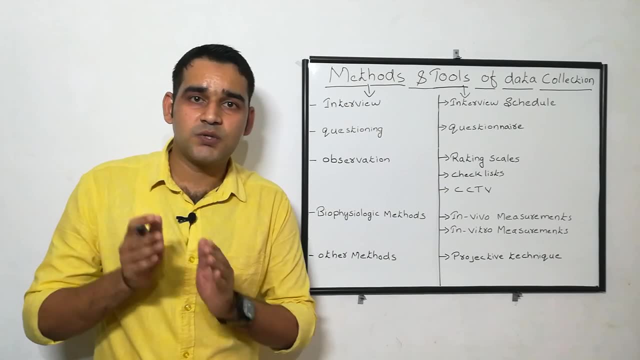 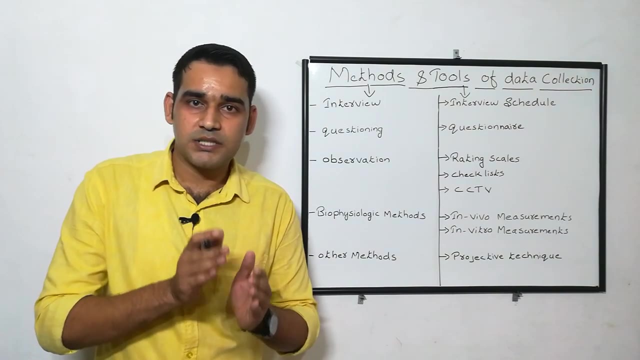 definition for rating scale is: it is a tool used to express the opinion of the performance of a person or a subject or a situation. it is a tool used to express the opinion or the the the the performance of a person or situation or a object got it. so the question will be: i will. 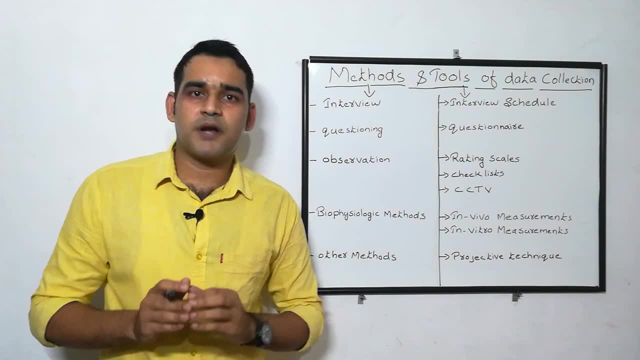 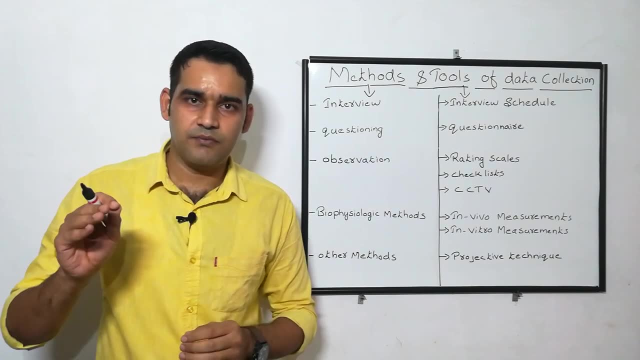 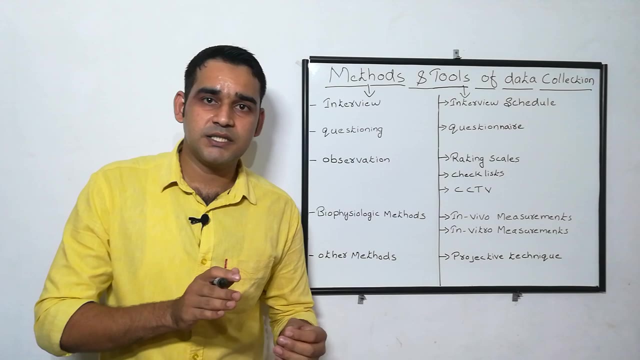 give you an example. the question will be: judge the performance of nurses in icu. the answer will be: very active, active, moderately active and passive. so you have to rate according to your view whether they are very active or they are active, or they are moderately active, or whether they are. 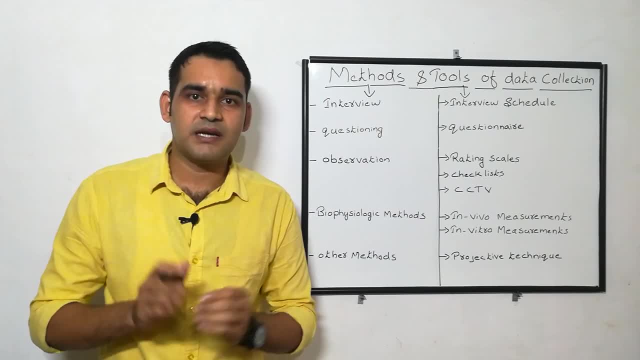 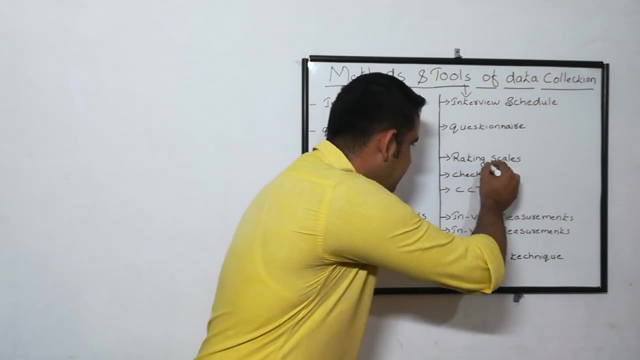 passive you have to write, got it. whether it is very good, good, poor or very poor like that, you have to write one thing, got it. it is very familiar to you. i think nowadays it is very popular. next one is checklist. checklist means from the name itself, you will get list. a list of items will be there and 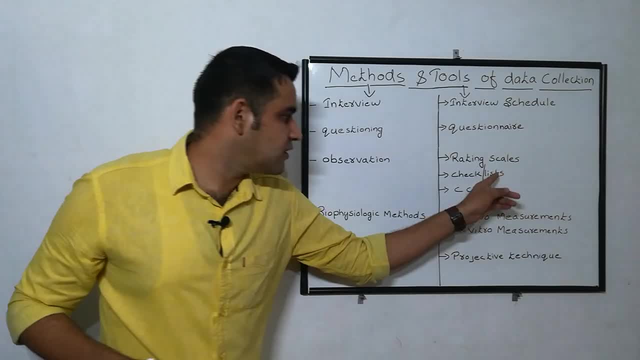 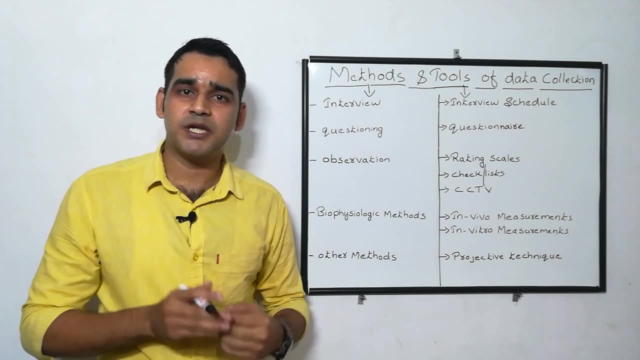 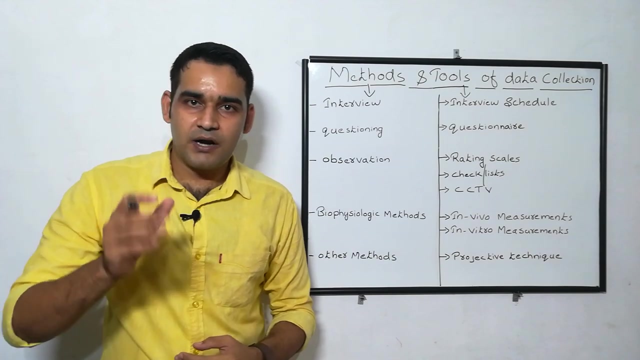 you will check it for its presence or not. a list of items will be there. you will check for it presence or not. Suppose a food inspector is coming to inspect a restaurant, So a list of items will be there, What are the things to inspect, and all regarding the purity of water. 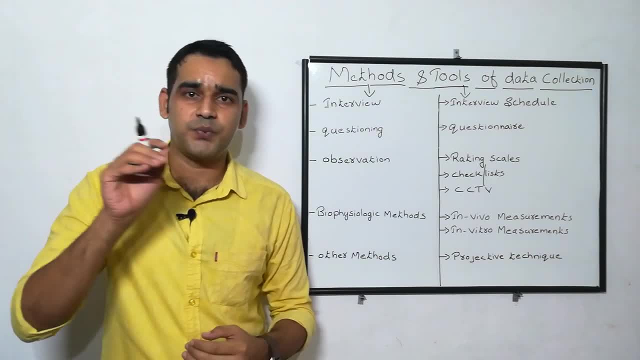 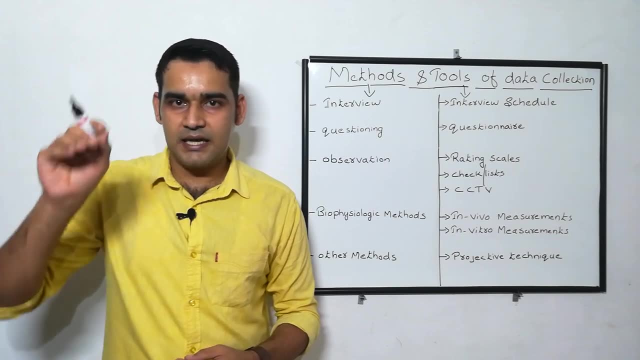 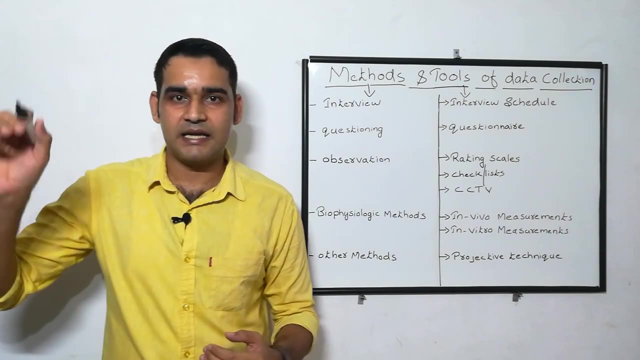 So he will check whether it is yes or no. whether it is pure or not, So he will take it. what it regarding the quality of food, next one, So he will take it whether it is yes or no, proper or not. What it regarding the behavior of the staff, So he will take yes or no. regarding the 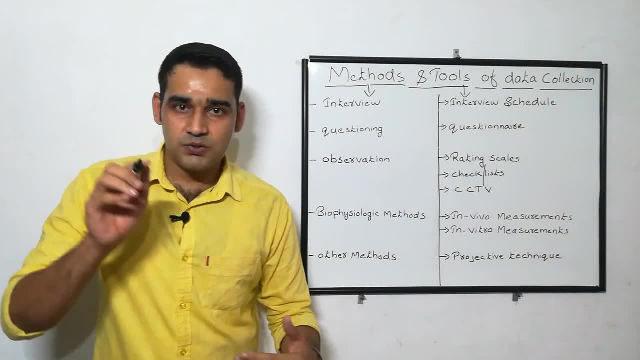 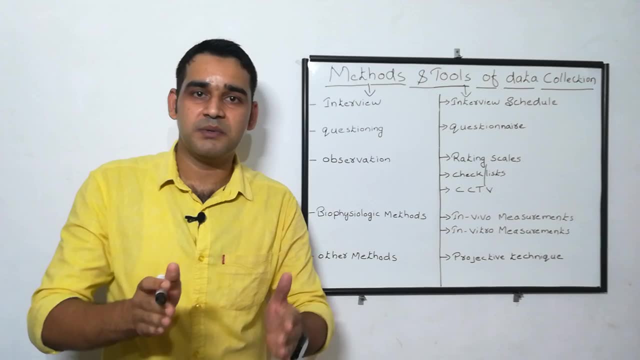 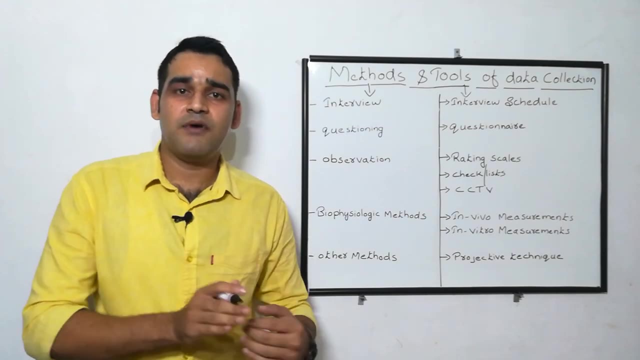 Electric supply, ventilation, drainage system. So it is proper or not. He will take it. Finally he will come to a conclusion. a list of items will be there already prepared list will be there. You will check for the presence or absence. Another example I can give that is a examiner's evaluating a nursing student. 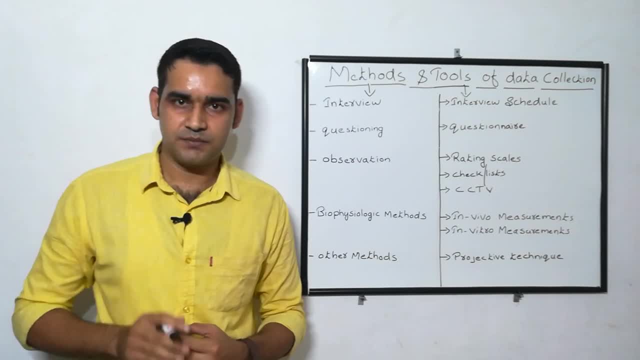 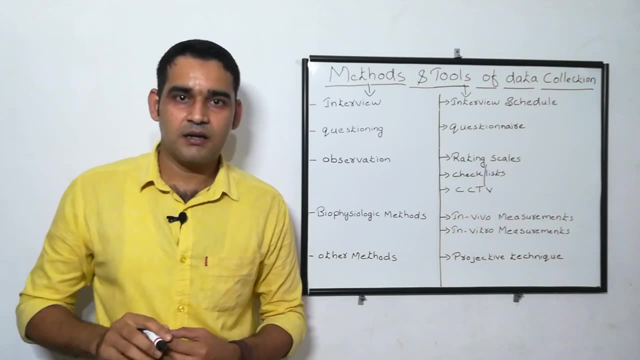 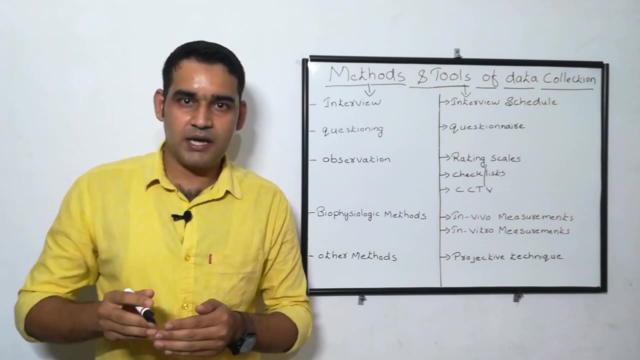 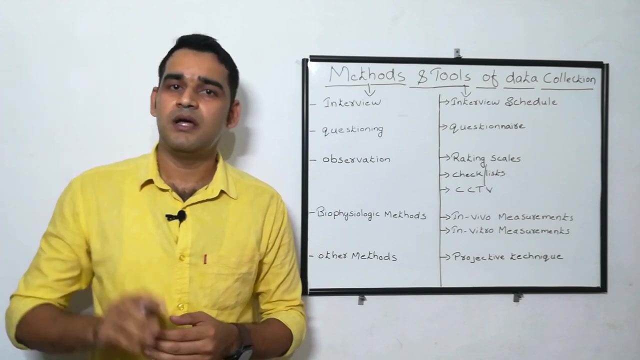 while performing blood pressure procedure. So the examiner will check whether hand washing done or not, So he will take Okay Next one. Next one is explain the procedure or not, articles arranged or not, Okay, documentation done or not Got it. So he will check it and finally he will come to a conclusion. 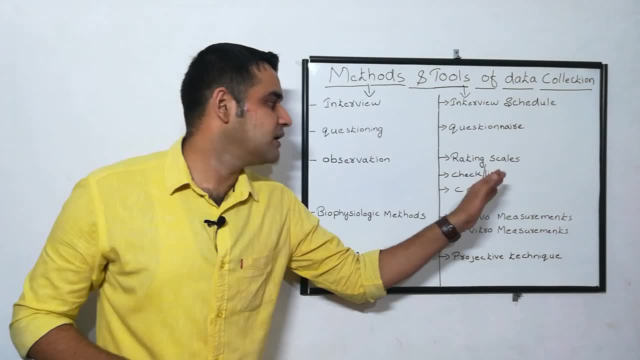 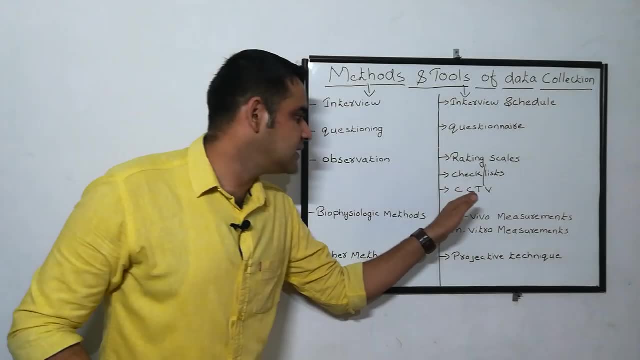 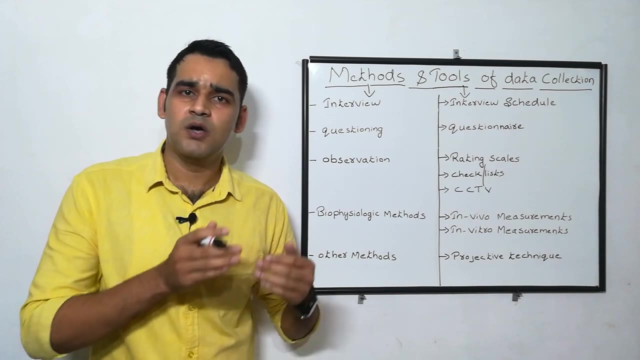 That is called checklist. a list of items will be there. He will check for the Whether the right is present or not. But it next one is CCTV. that is closed circuit TV. That is camera using camera using CCTV. the Observer will observe it is also very familiar nowadays. 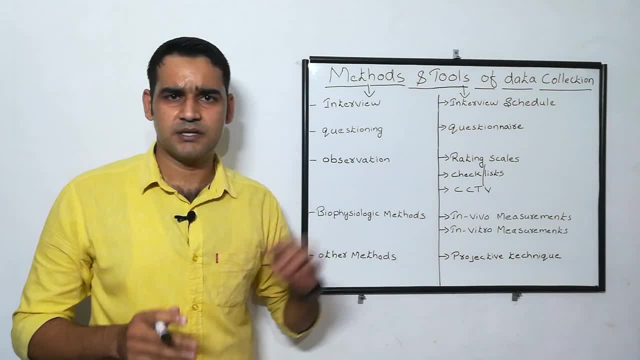 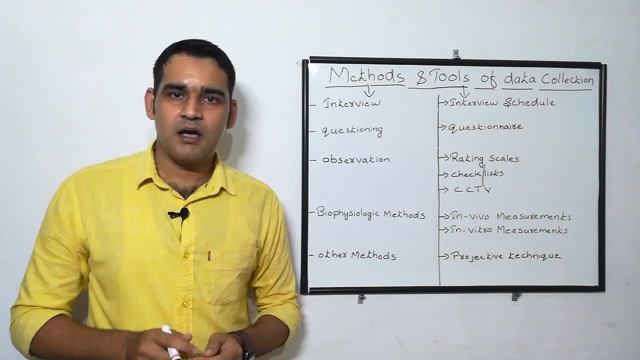 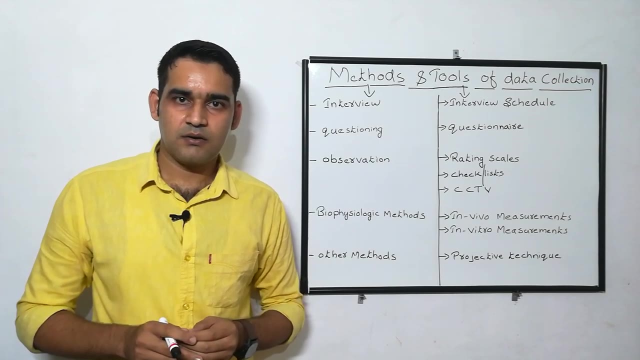 Okay, so no need of explanation regarding cctv observation. What it next one is Biophysiological methods. Biophysiological methods means nothing. you are checking the biological as well as the physiological status of the subject. Quote it: that means: regarding the blood pressure, what is happening in the body, That is physiological aspect as well as the biological aspect. data is not reliable, Is not like the machine using to study the curry while reading a book. 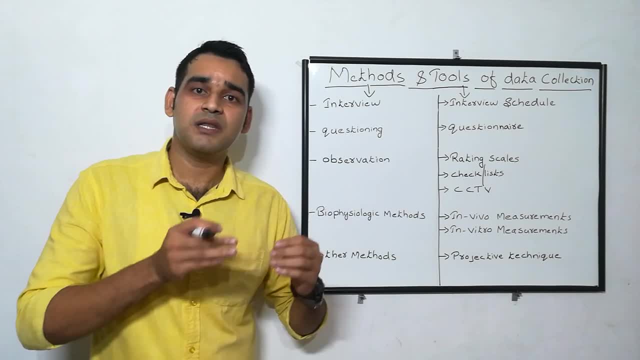 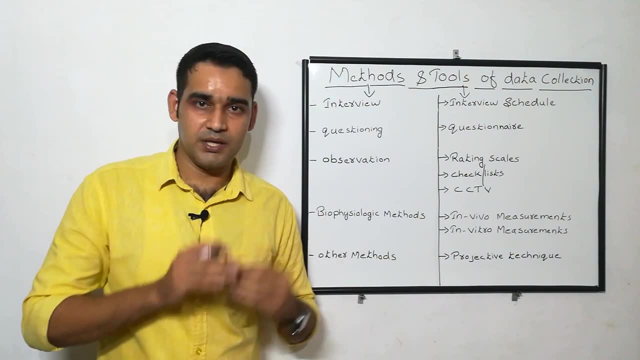 That means, regarding the blood pressure, What is happening in the body- That is, physiological aspect as well as the biological aspects. What is happening internally in the body? You are checking. That is a method. So the tool used for biophysiological method is in vivo measurement. 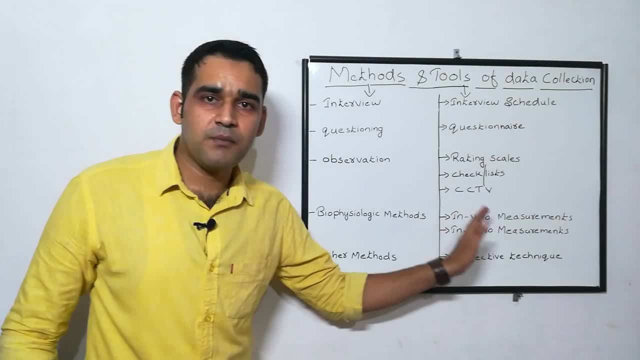 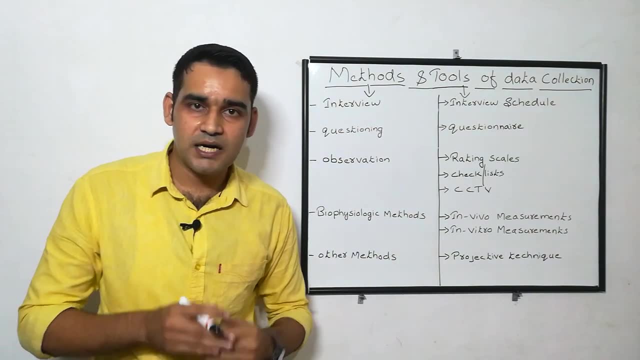 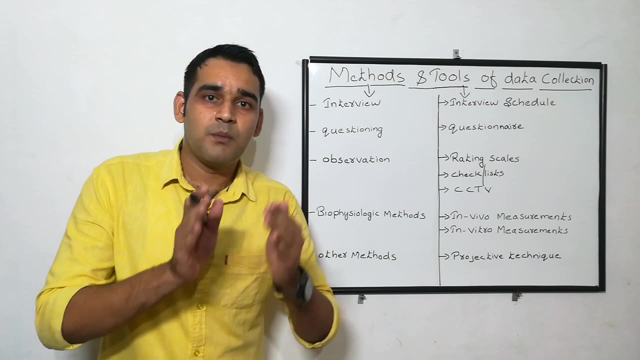 as well as in vitro measurement. In vivo measurement as well as in vitro measurement: In vivo measurement means the procedure is done and the measurement is done within the body. only The procedure is done, as well as keep it in mind, as well as measurement is done within the body. 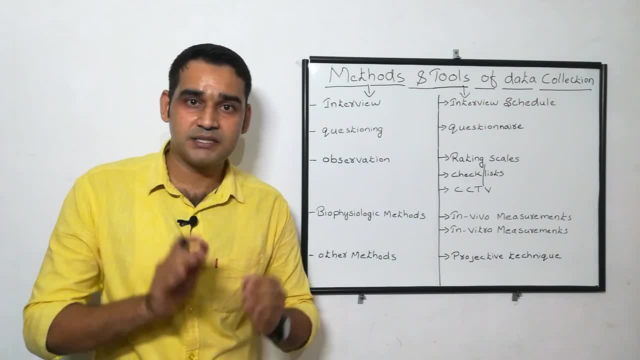 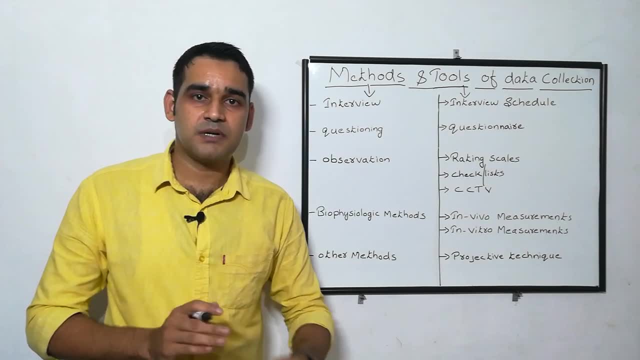 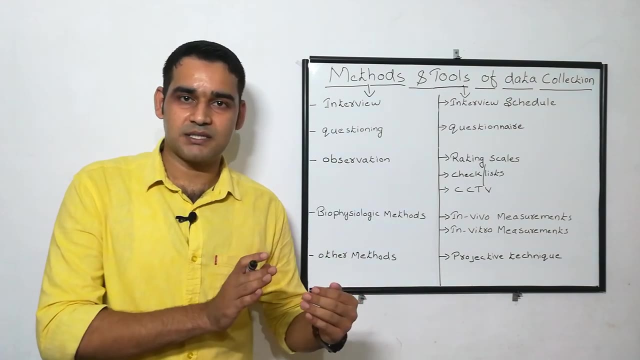 only. That means while checking blood pressure. best example is checking BP for in vivo measurement. Checking blood pressure, the measurement as well as the procedure is done within the body only and measurement is done from same place. only Got it Checking temperature. That is also a good example for in vivo measurement. Maybe you will get confusion. 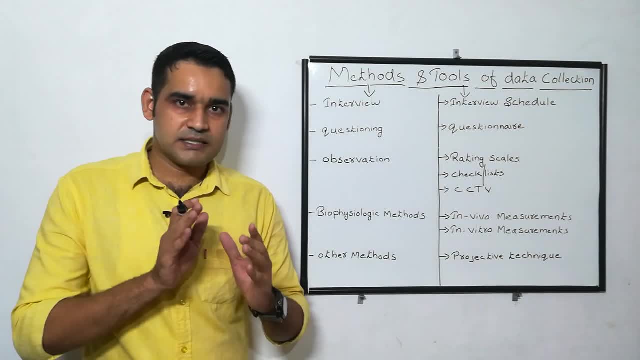 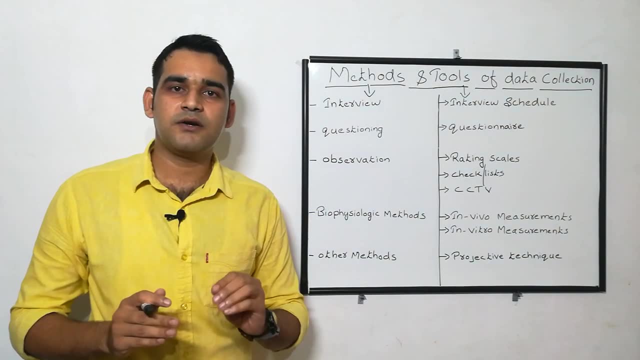 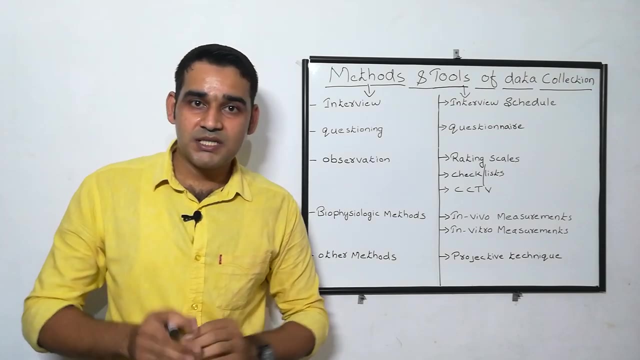 While I am explaining regarding in vitro, you will get the exact idea regarding these two methods. In vitro measurement means listen carefully. in vitro measurement means procedure is done and measurement is done outside the body. Procedure is done and measurement is done outside the body. That is blood test or urine test.